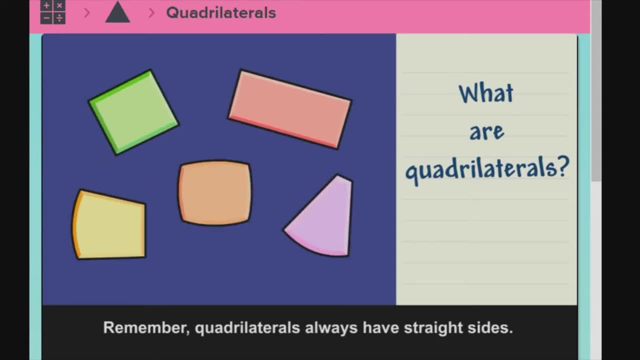 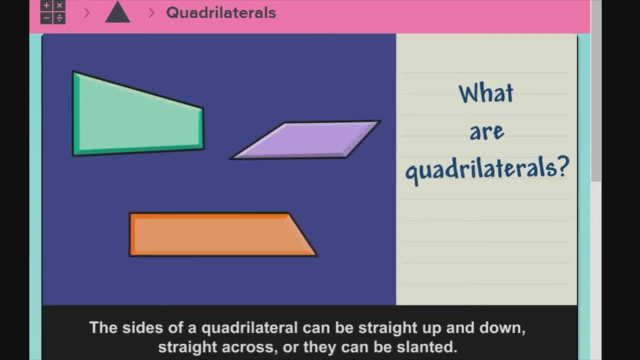 Remember, quadrilaterals always have straight sides, So these shapes aren't quadrilaterals. The sides of a quadrilateral can be straight up and down, straight across, or they can be slanted. What did the quadrilateral say to the empty room? 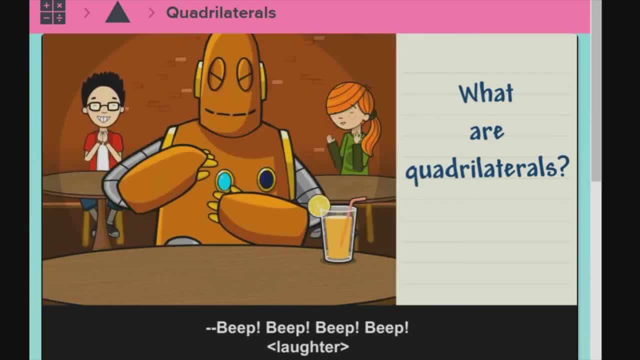 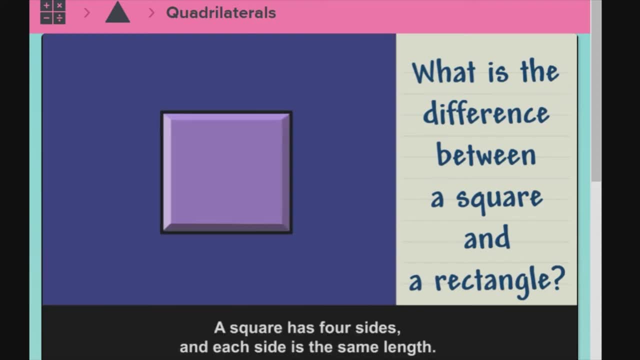 Square is everybody. It says. if a square becomes square it's the same length as a rectangle. How many colors are there in a square? Four colors and four sides. Five colors, Three colors- CrYeDs- A square is set after a ball of hair, so there can be either four or eight colors. 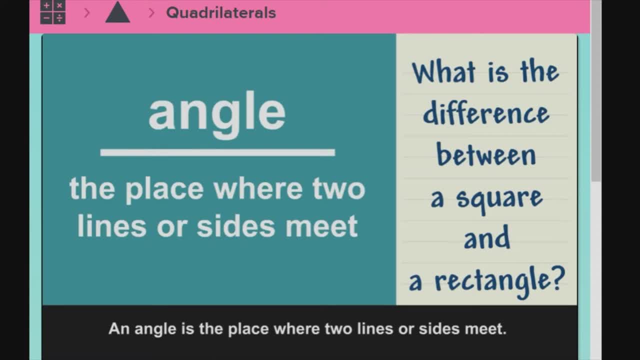 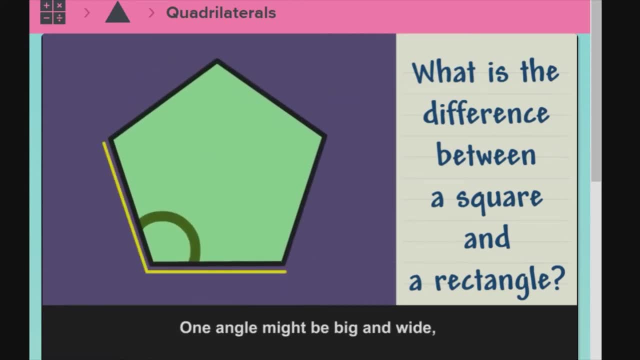 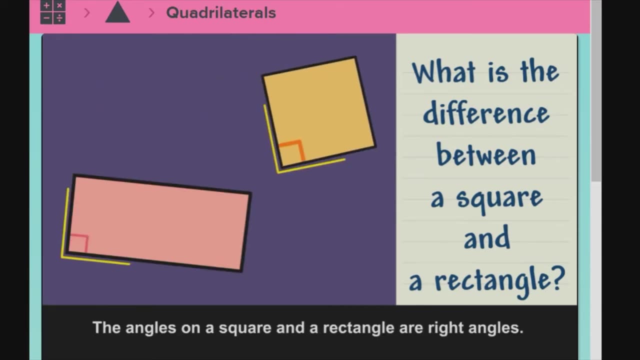 A square has six, Five colors. One square is slanted, A rectangle is slanted, Beautiful, Sweet. One angle might be big and wide and another might be narrow and small. The angles on a square and a rectangle are right angles. 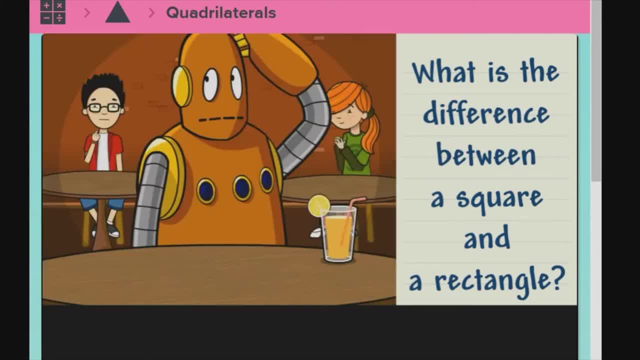 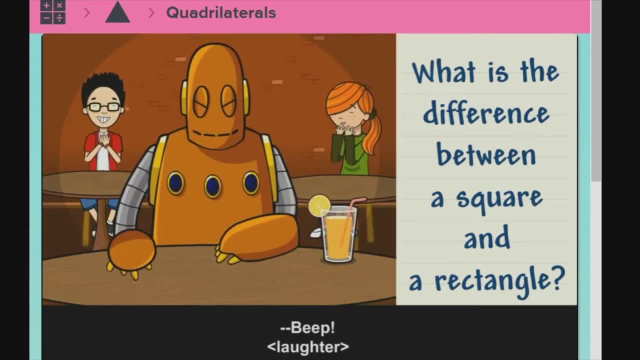 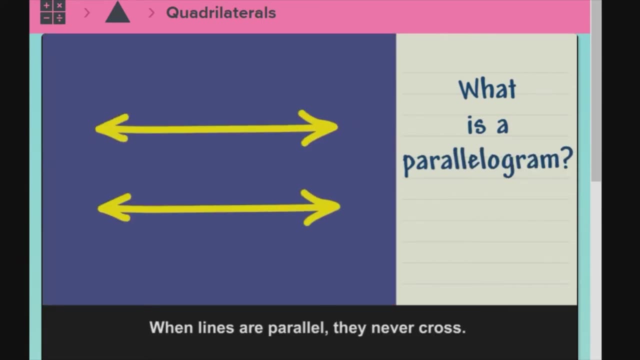 Why did the square miss class? Because she sprained her angle. What is a parallelogram? When lines are parallel, they never cross. The distance between them is always the same, no matter where you measure. This quadrilateral has one pair of parallel sides. 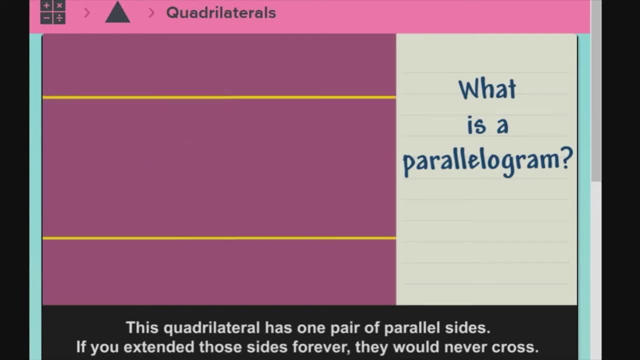 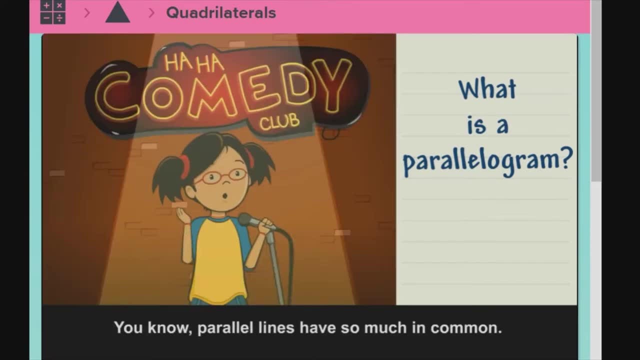 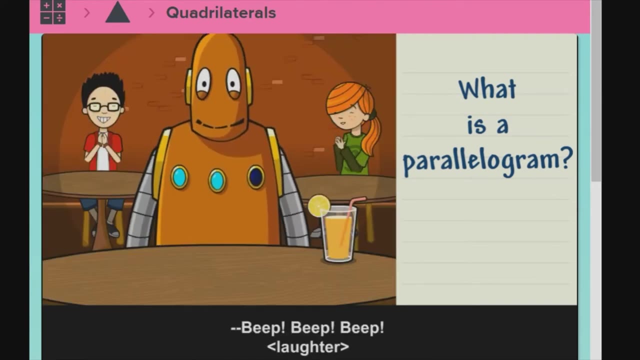 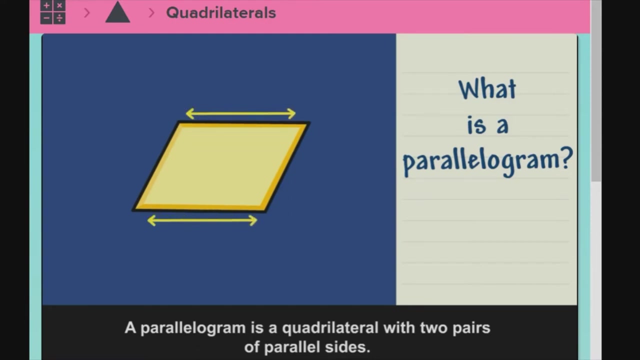 If you extended those sides forever they would never cross. But this quadrilateral does not have any parallel sides. You know, parallel lines have so much in common. It's a shame they'll never meet. A parallelogram is a quadrilateral with two pairs of parallel sides. 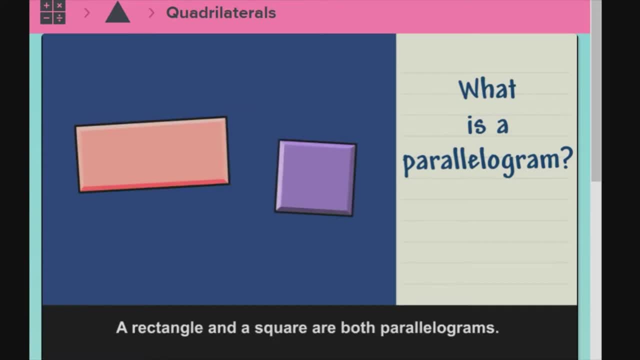 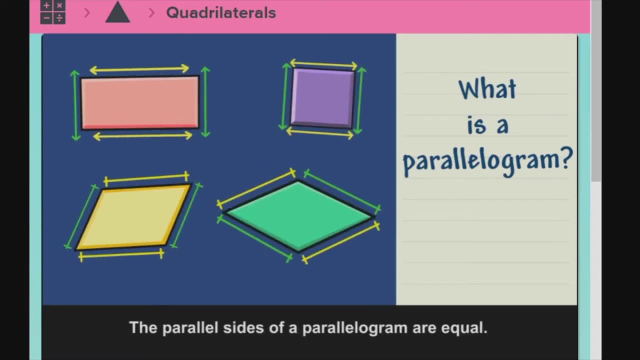 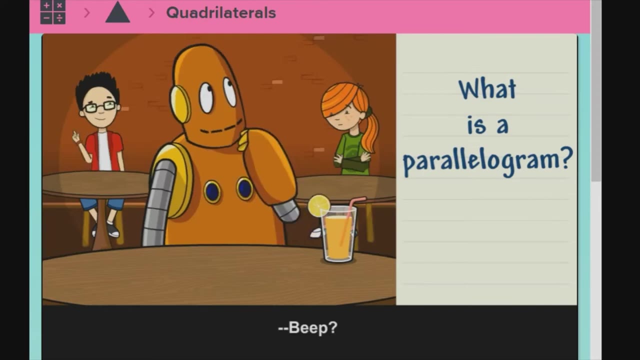 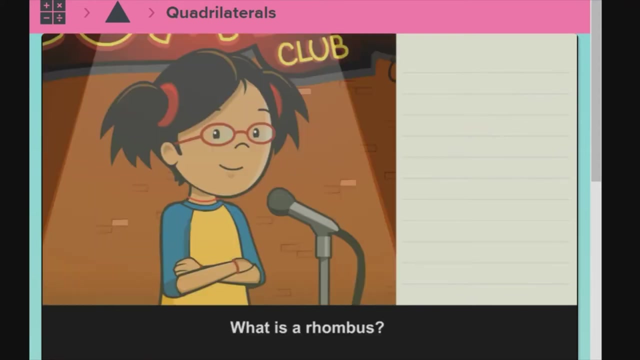 A rectangle and a square are both parallelograms. They each have two pairs of parallel sides. The parallel sides of a parallelogram are equal. Why did the parallelogram go jogging? So it could stay in shape. What is a rhombus? 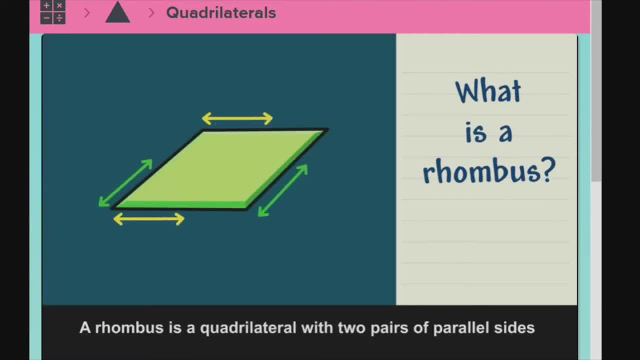 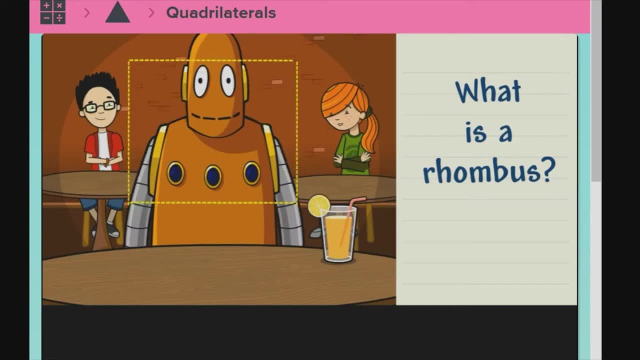 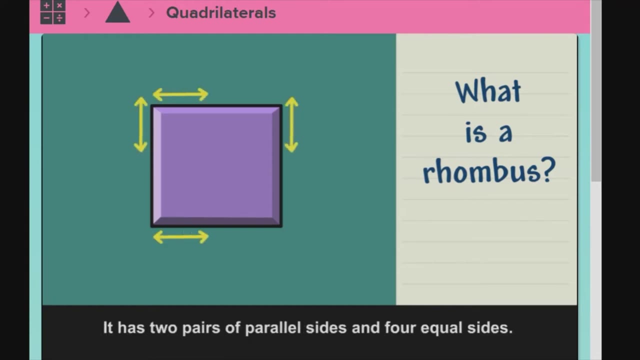 A rhombus is a quadrilateral with two pairs of parallel sides and four equal sides. Right, Moby A square is also a rhombus. It has two pairs of parallel sides and four equal sides. A rhombus, square and rectangle are all parallelograms. 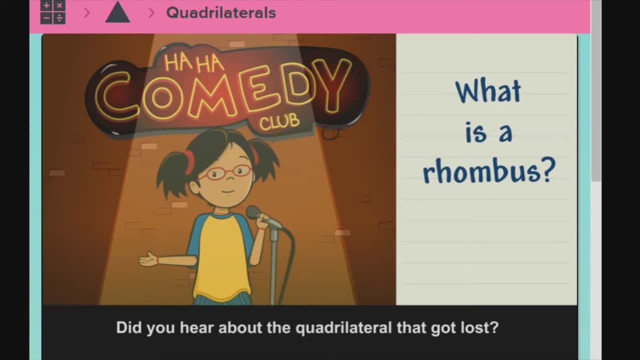 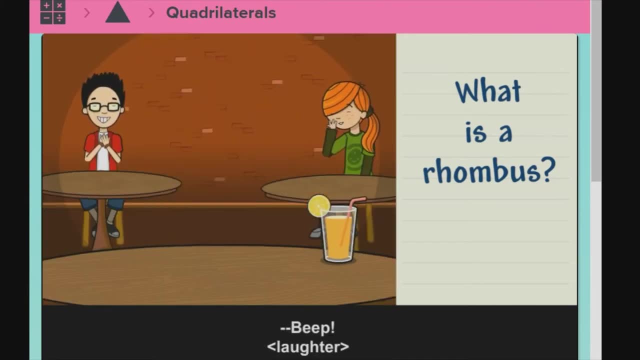 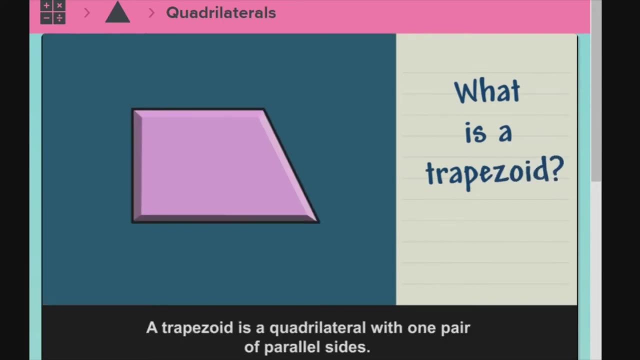 Did you hear about the quadrilateral that got lost? It took the wrong bus. What is a trapezoid? A trapezoid is a quadrilateral with one pair of parallel sides. A trapezoid can be a quadrilateral with two pairs of parallel sides. 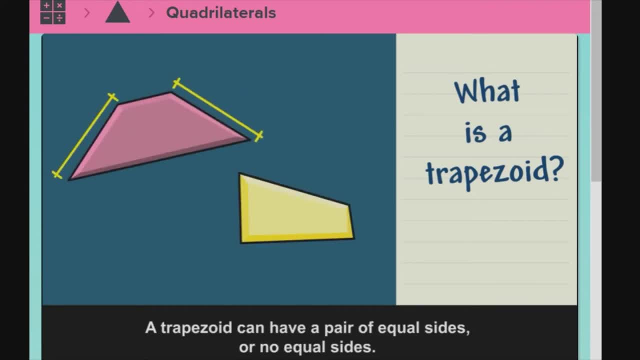 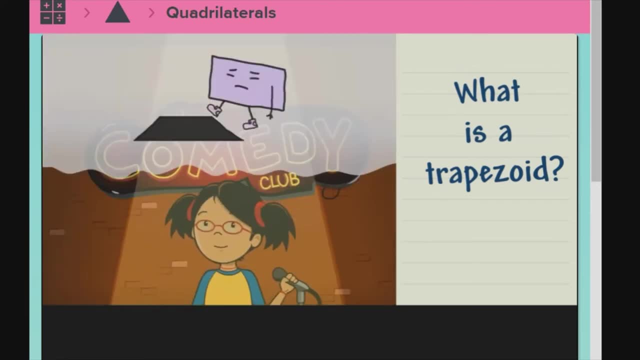 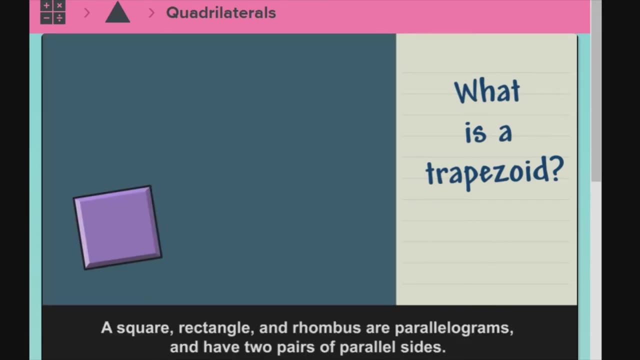 A trapezoid is a quadrilateral with one pair of parallel sides. A trapezoid can have a pair of equal sides or no equal sides. How do you catch a quadrilateral? You use a trap-o-zoid, A square. rectangle and rhombus are parallelograms and have two pairs of parallel sides. 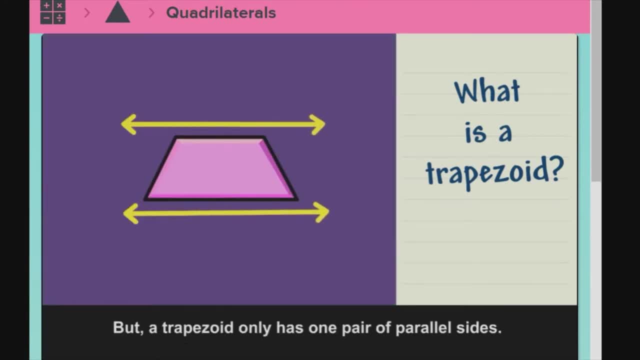 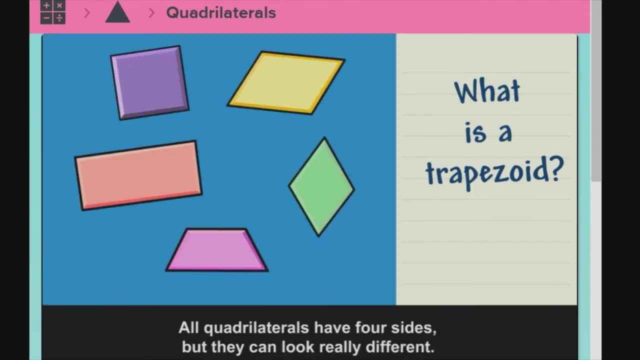 But a trapezoid only has one pair of parallel sides. You're right, Moby, All quadrilaterals have four sides, but they can look really different. Their sides and angles show how they're alike and different. What did one quadrilateral say to the other? 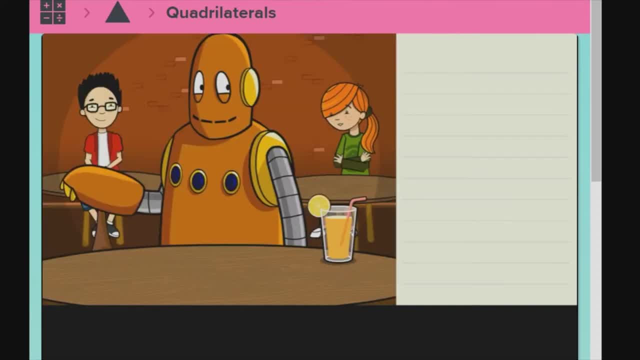 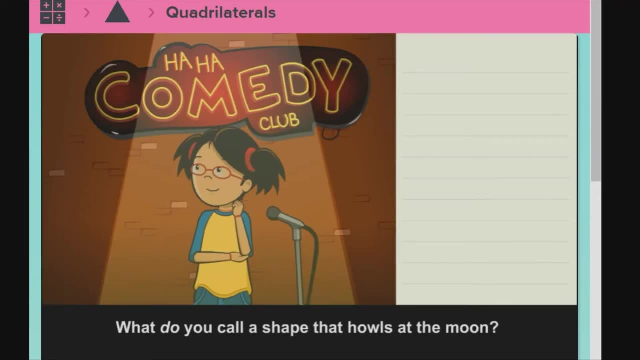 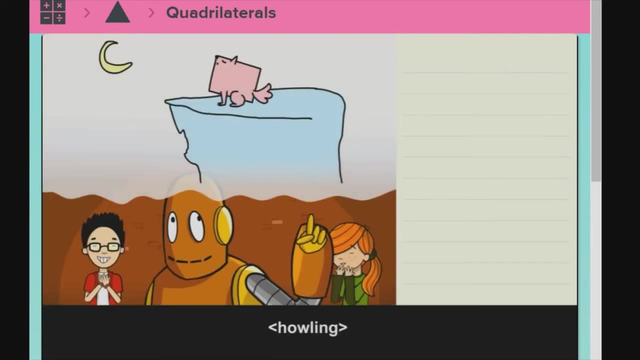 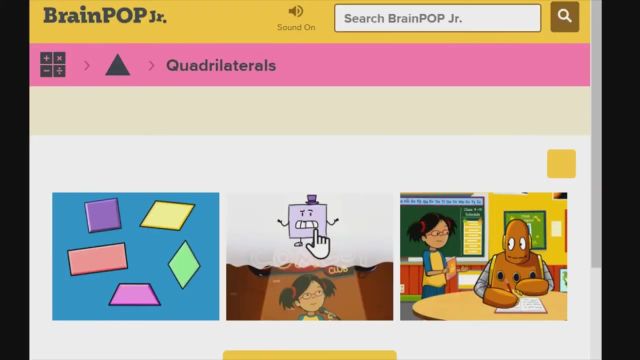 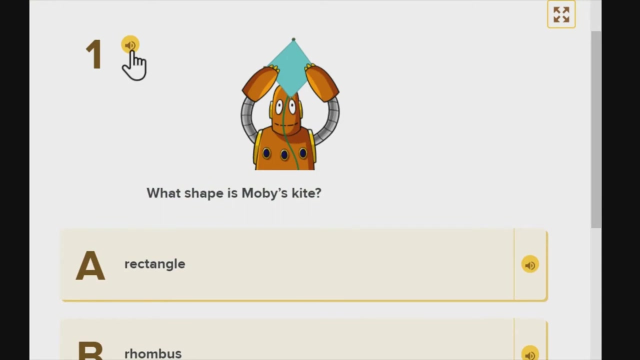 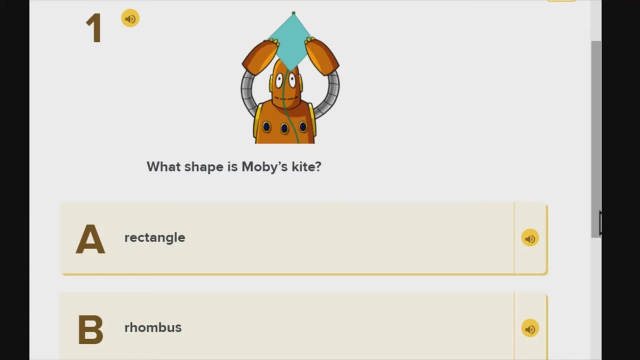 What side are you on? You have a joke. Let's hear it. What do you call a shape that howls at the moon? A square wolf, Start, Start. What shape is Moby's kite? Rectangle, Rhombus. 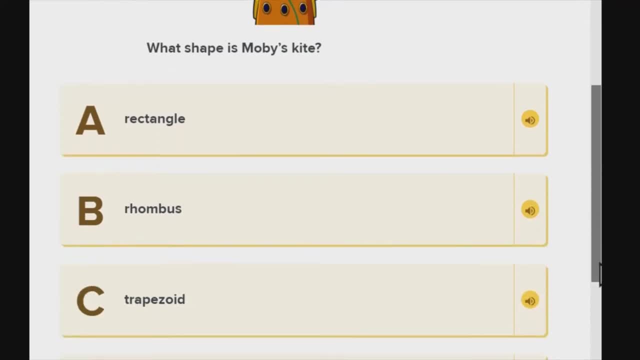 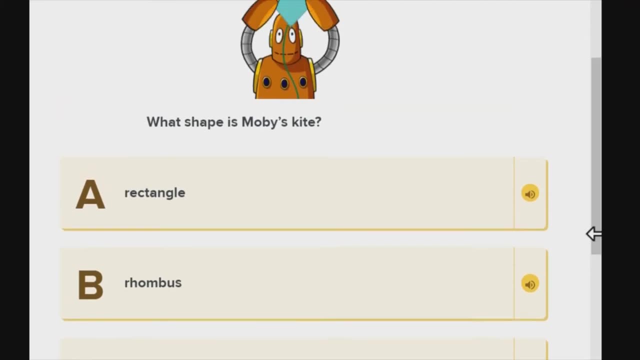 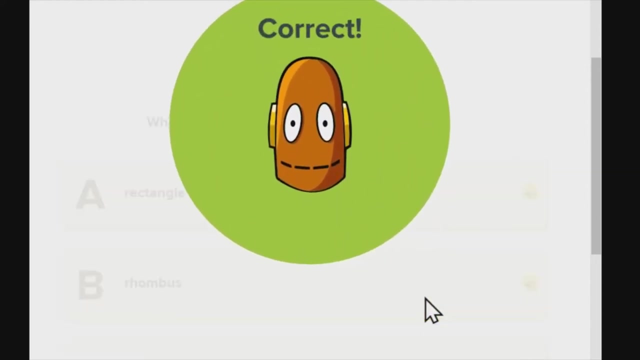 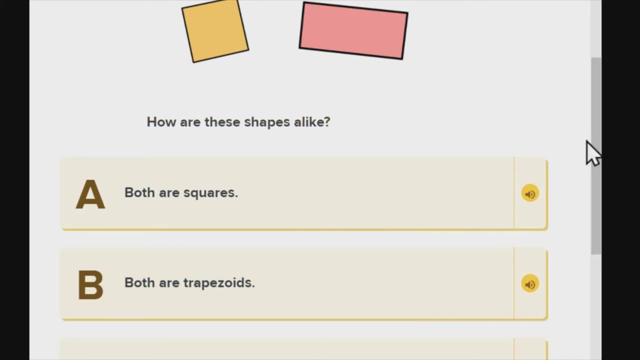 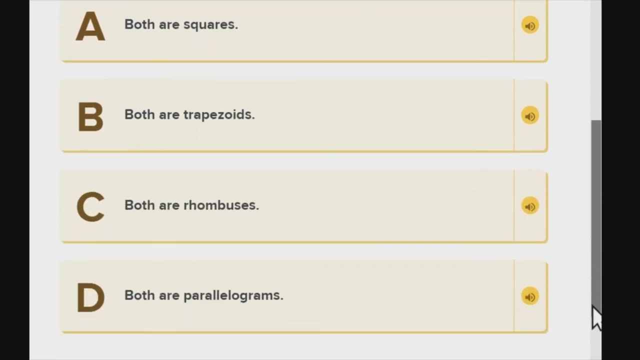 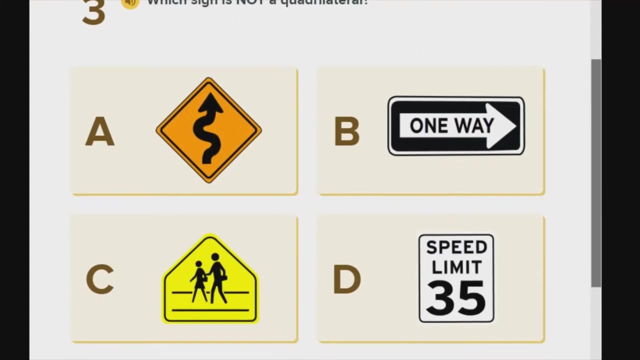 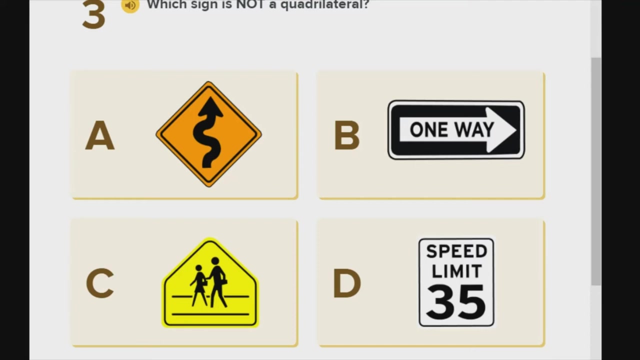 Trapezoid Triangle. How are these shapes alike? Both are squares, Both are squares, Both are trapezoids, Both are rhombuses, Both are parallelograms. Which sign is not a quadrilateral, Quadrilateral, Quadrilateral? 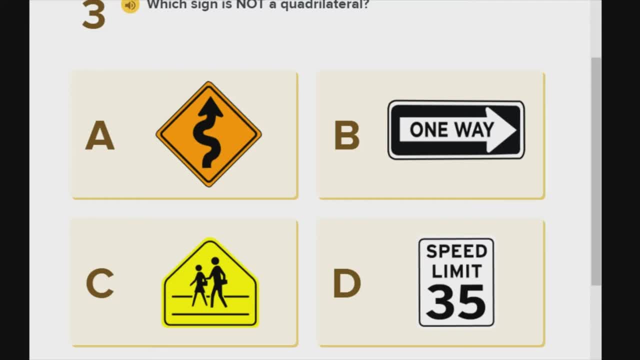 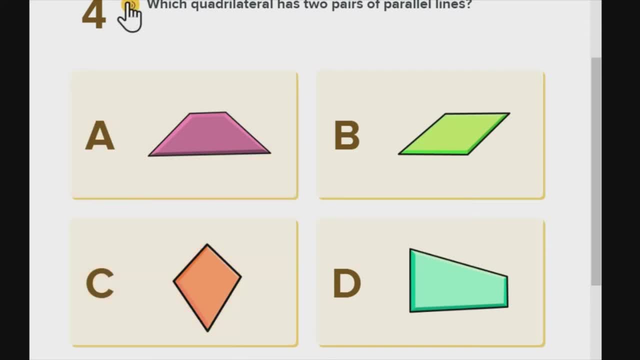 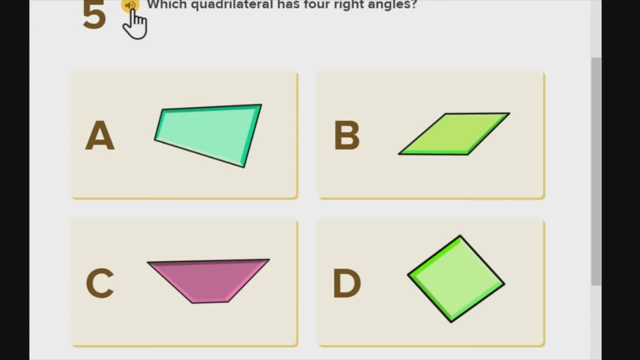 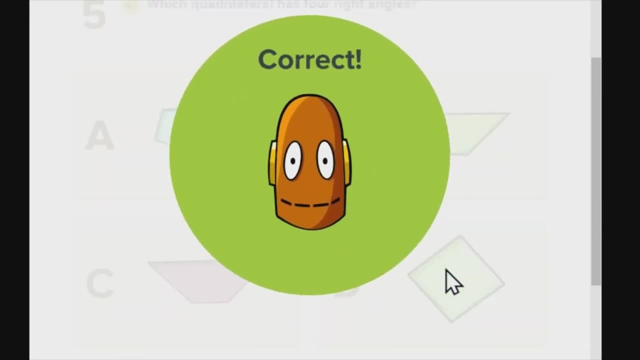 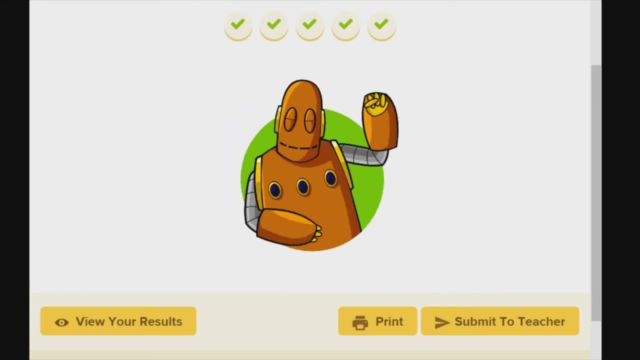 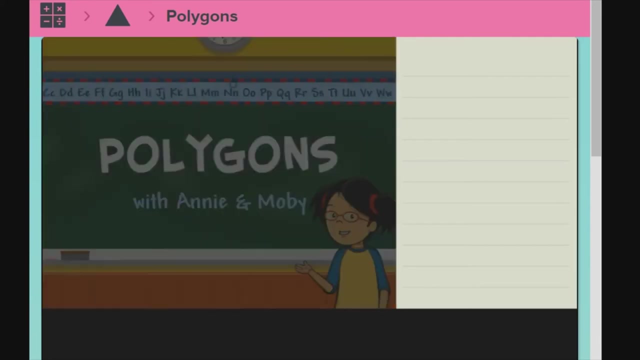 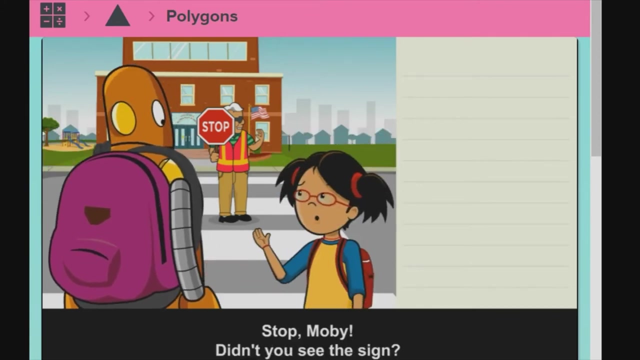 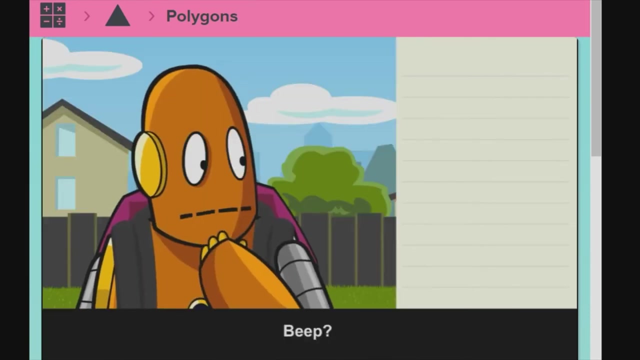 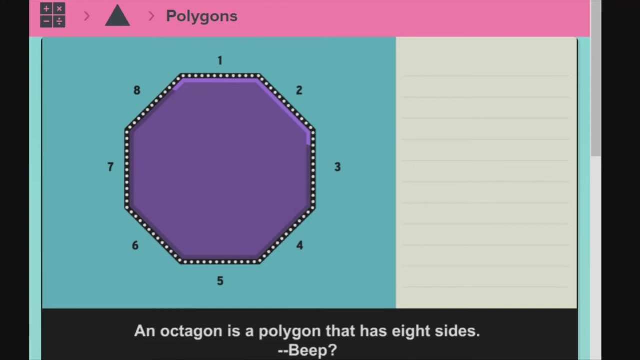 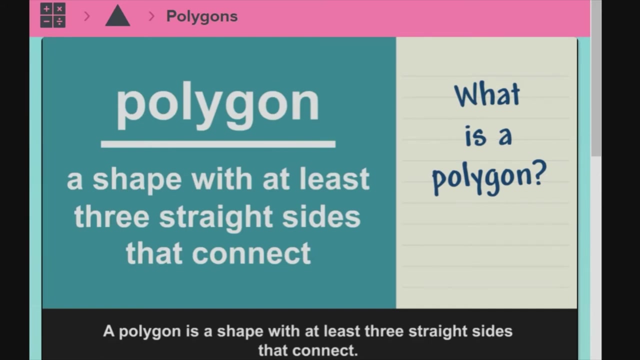 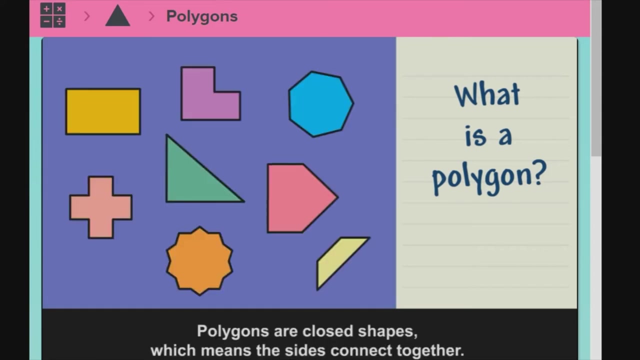 Which quadrilateral has four right angles? The quadrilateral has four right angles. There is a polygon that has eight sides. What is a polygon? A polygon is a shape with at least three straight sides that connect. Polygons are closed shapes, which means the sides connect together. 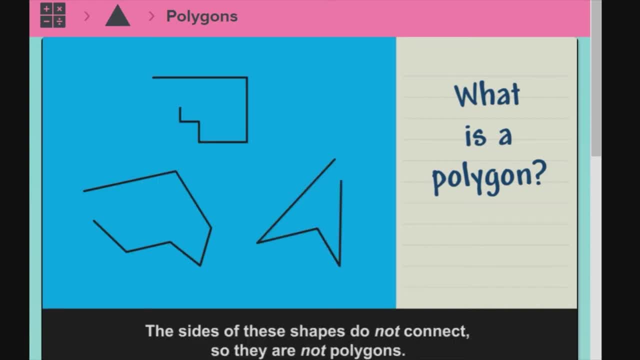 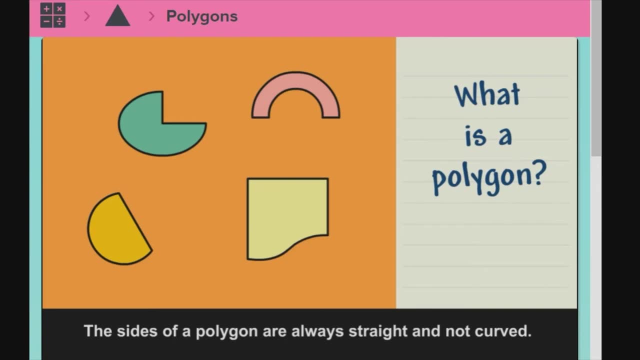 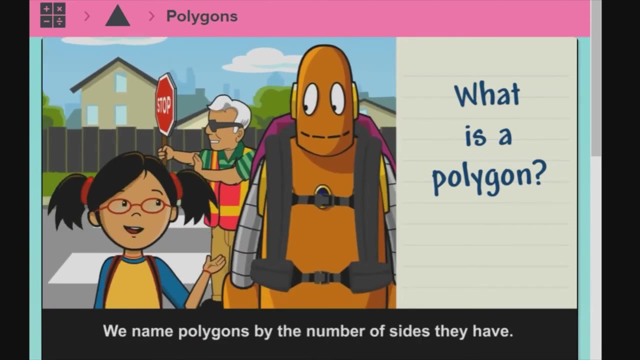 The sides of these shapes do not connect, so they are not polygons. The sides of a polygon are not polygons. Polygons are always straight and not curved, so these aren't polygons either. We name polygons by the number of sides they have. 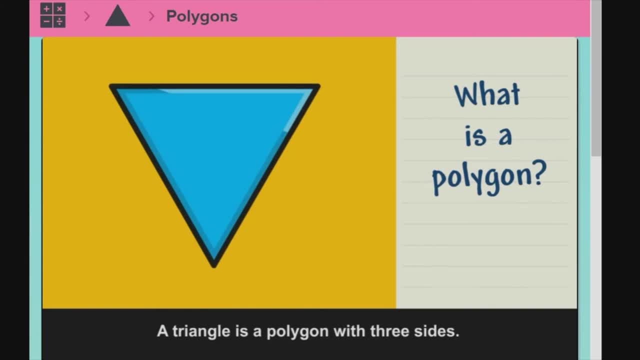 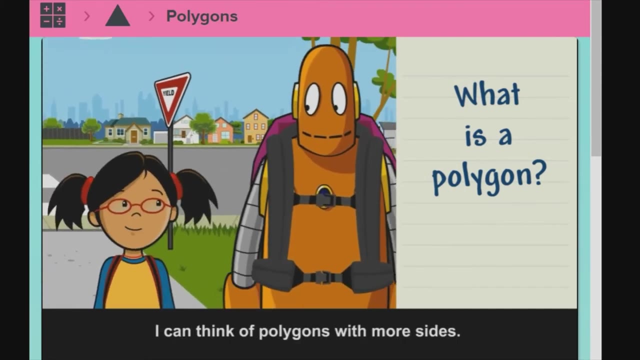 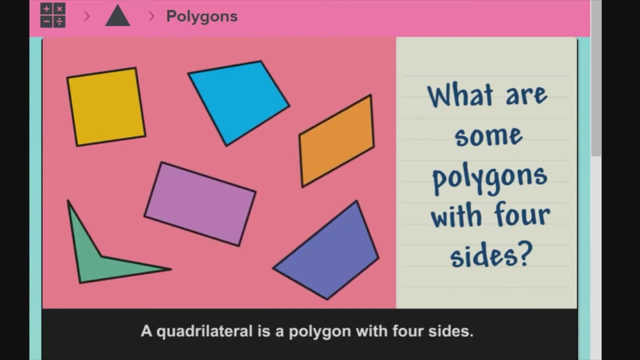 A triangle is a polygon with three sides. A vertex is the point where the sides come together. A triangle has three vertices. I can think of polygons with three sides. What are some polygons with four sides? A quadrilateral is a polygon with four sides. 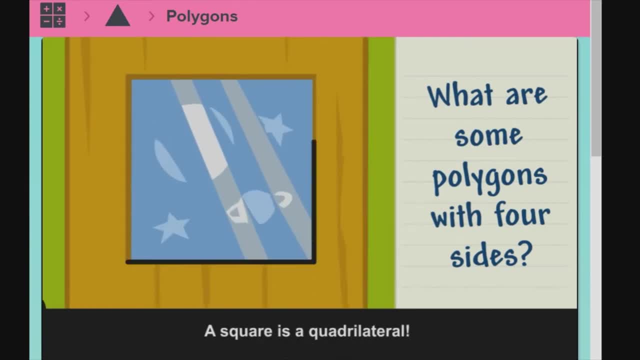 Right, Moby, A square is a quadrilateral. It has four sides that are equal or the same size. A square has four vertices. A rectangle is also a quadrilateral. It has four sides and four vertices, just like a square. 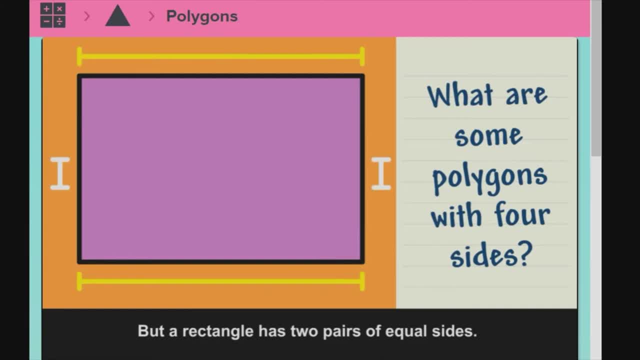 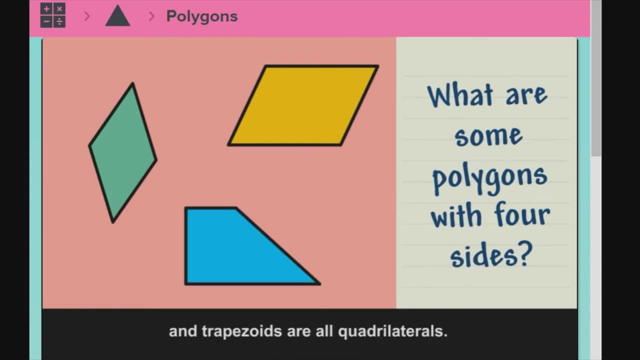 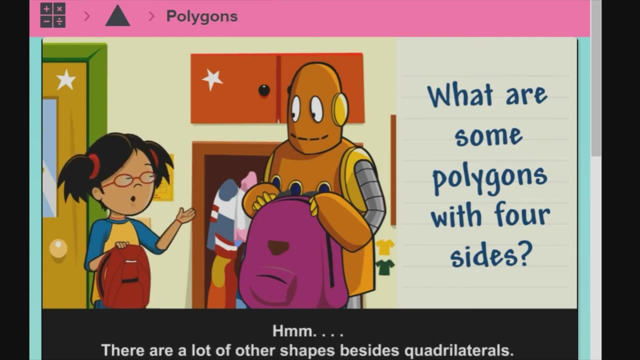 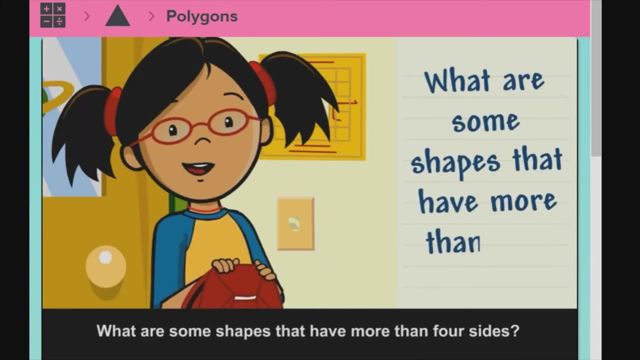 But a rectangle has two pairs of equal sides. Rhombuses, parallelograms and trapezoids are all quadrilaterals. Hmm, There are a lot of other shapes besides quadrilaterals. What are some shapes that have more than four sides? 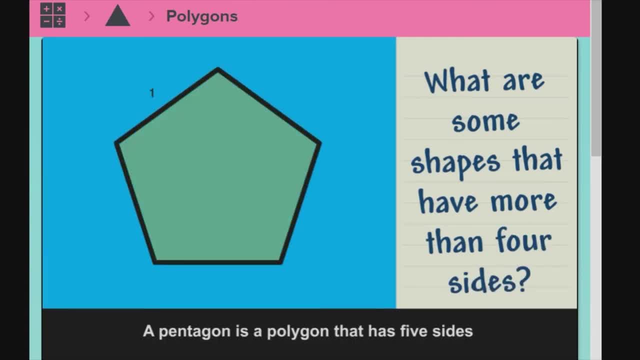 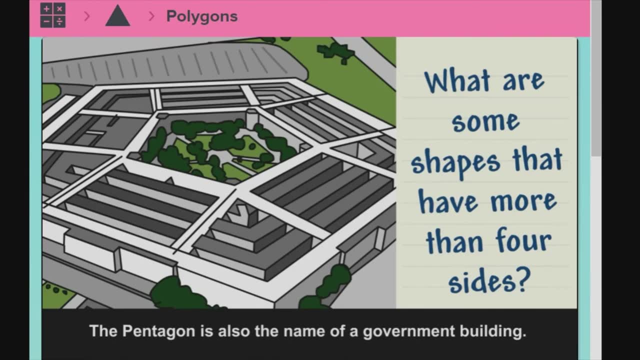 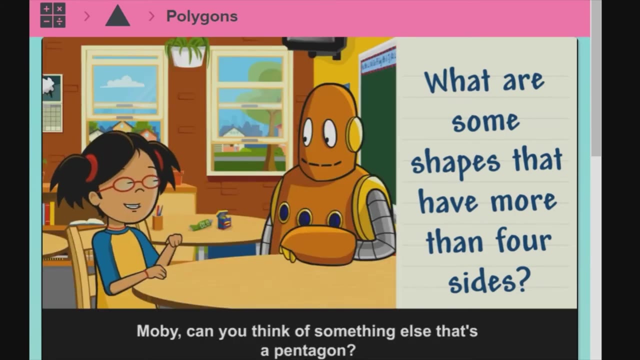 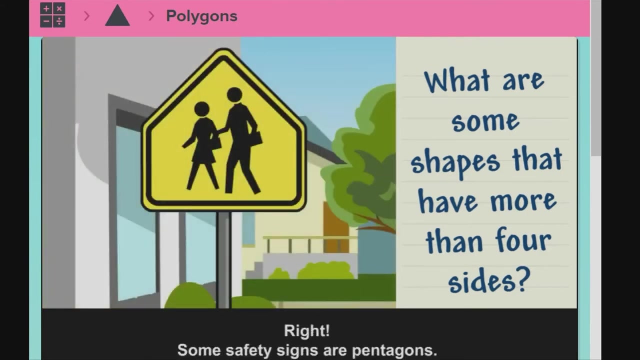 A pentagon is a polygon that has five sides and five vertices. The pentagon is also the name of a government building. You can see why, Moby. can you think of something else? that's a pentagon, Right? Some safety signs are pentagons. 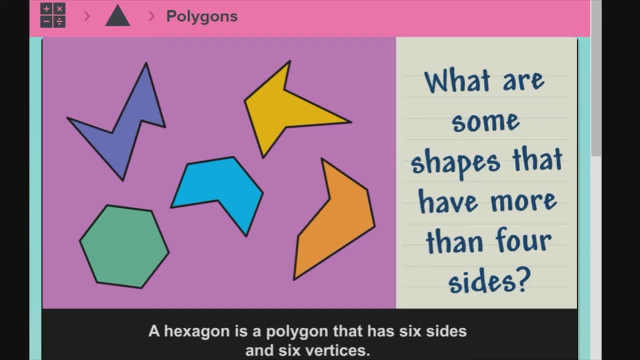 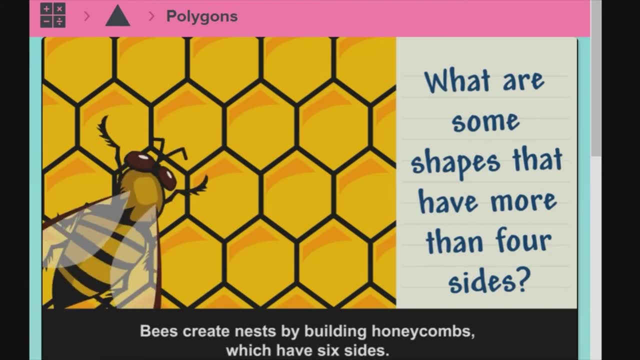 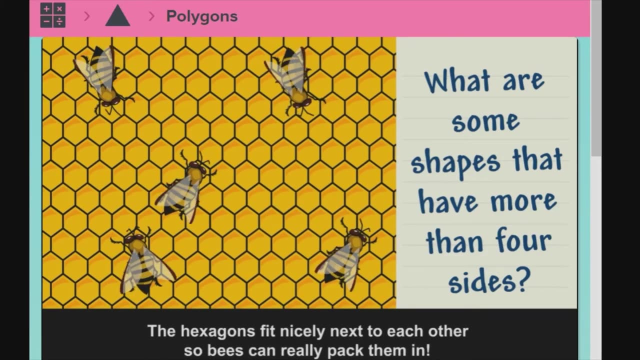 A hexagon is a polygon that has six sides and six vertices. Bees create nests by building honeycombs which have six sides. The hexagons fit nicely next to each other, so bees can really pack them in. Can you think of something that's a hexagon? 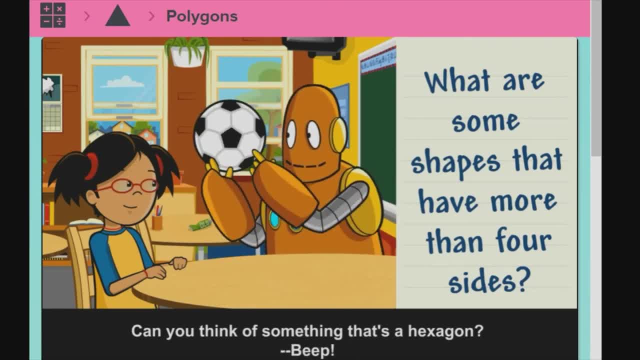 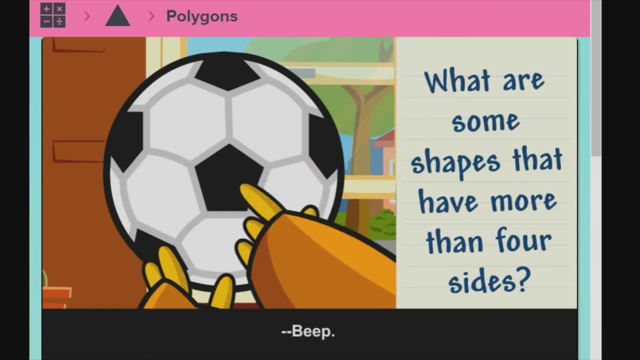 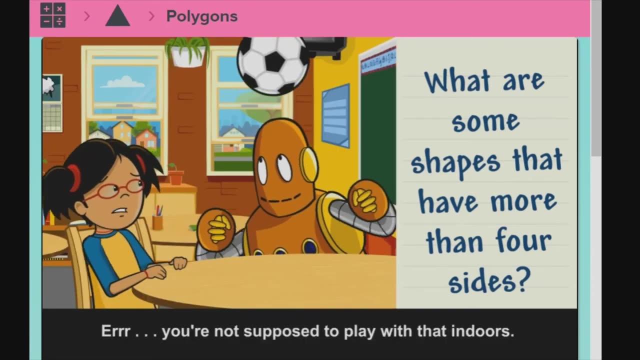 Right On this soccer ball. the white patches are hexagons, Oh, and the black patches are pentagons. Err, you're not supposed to play with that indoors, Uh-oh, Uh. moving on, A heptagon is a polygon that has seven sides and six vertices. 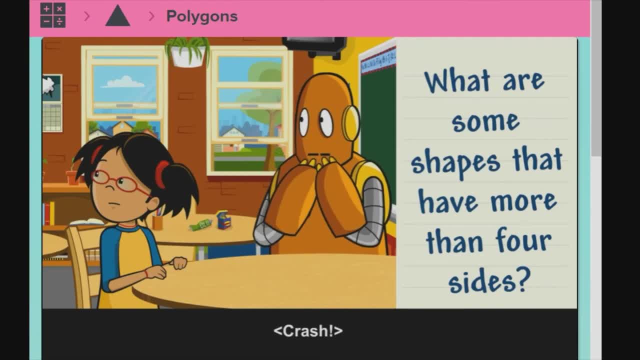 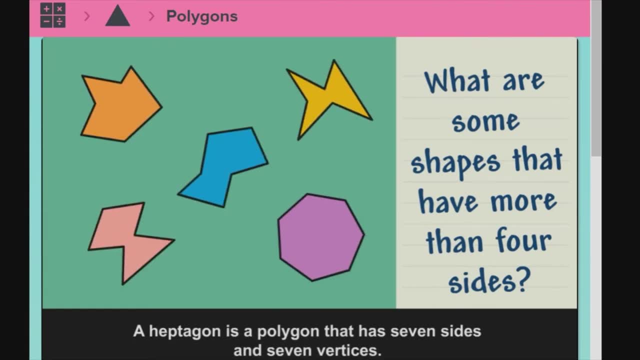 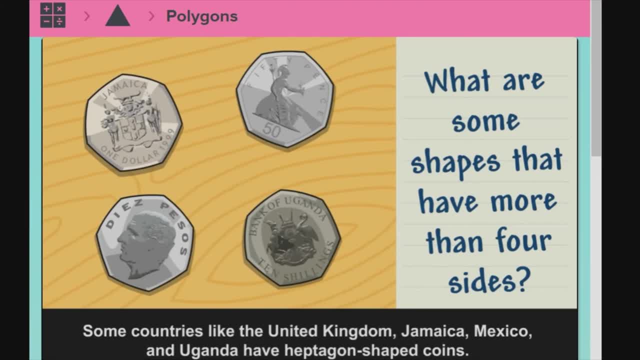 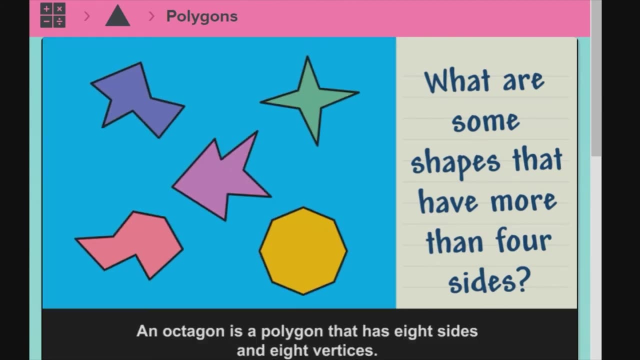 Bees create nests by building honeycombs which have six sides and six vertices. Cool: Some countries like the United Kingdom, Jamaica, Mexico and Uganda have heptagon-shape coins. An octagon is a polygon that has 8 sides and 8 vertices. 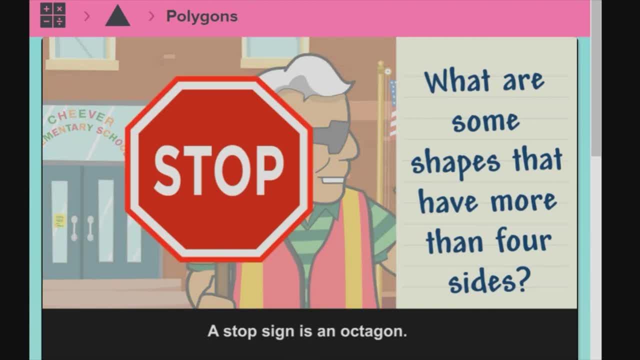 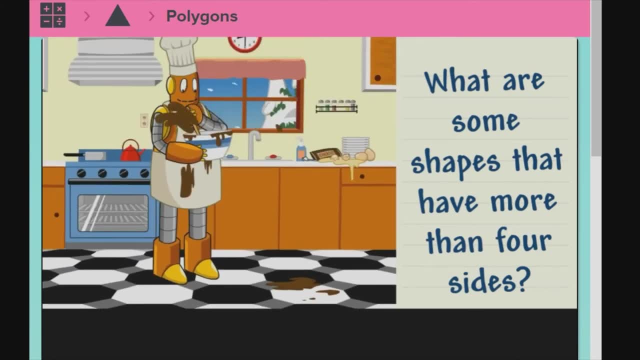 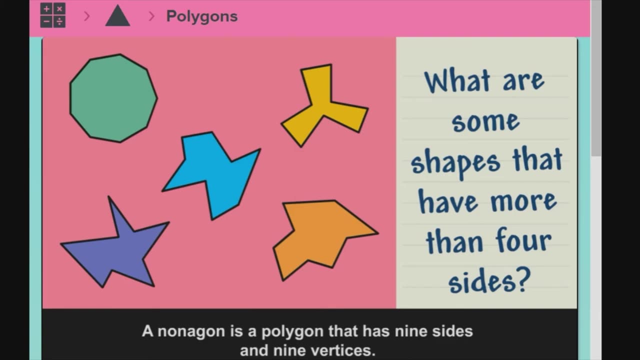 A stop sign is an octagon. Some of the tiles on our kitchen floor are octagons too. That is a very easy explain. A nonagon is a polygon that has nine sides and nine vertices. Hmm, I can't think of anything that has nine sides. 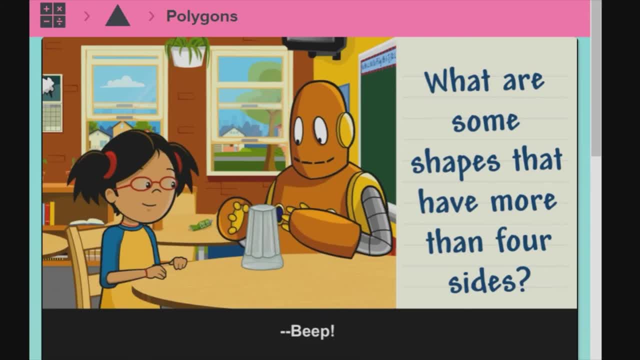 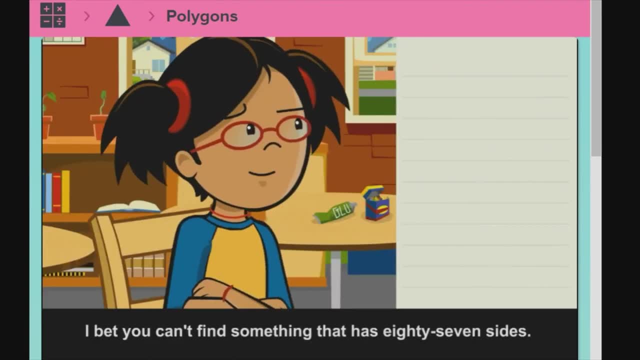 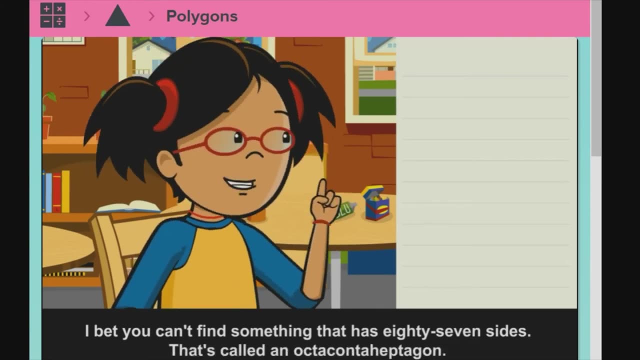 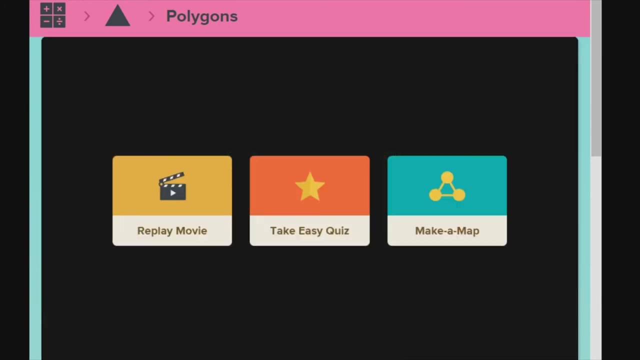 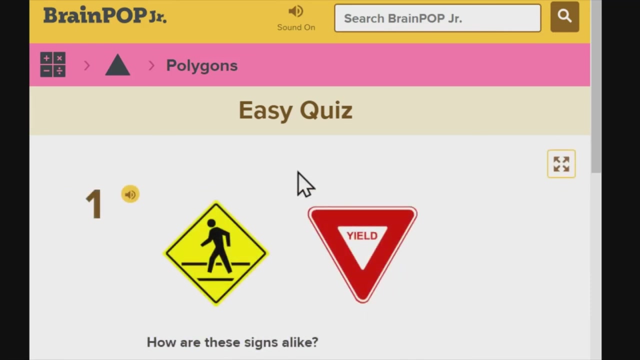 Can you, Moby Whoa, check it out? This glass is a nonagon. I bet you can't find something that has 87 sides. That's called an octacontaheptagon Start. How are these signs alike?